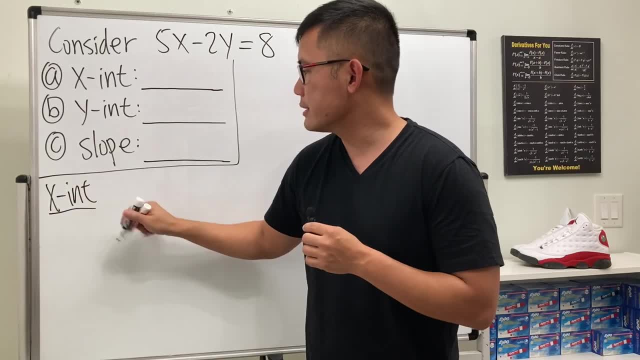 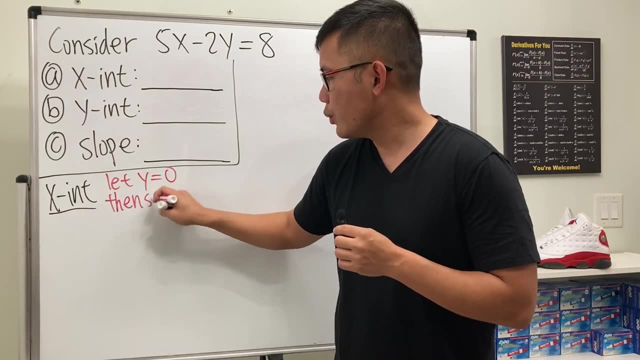 So right here, for the x-intercept, what we have to remember is we have to let y to be 0, and then after that we will be solving for x. So this, right here, is the key, and you just have to remember. 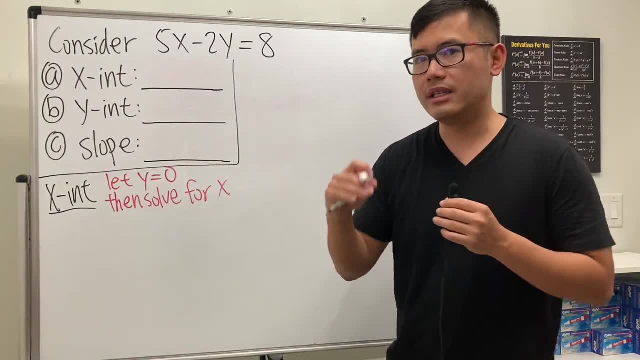 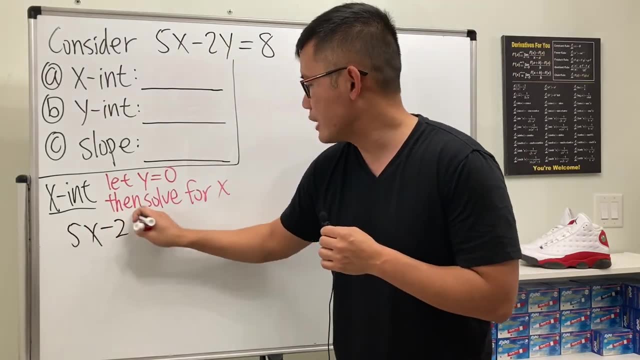 for x-intercept, you let y equal to 0, because it's on the x-axis. So let's go ahead and just put 0 into here and we will get 5x-2x0, and that will be equal to 8.. 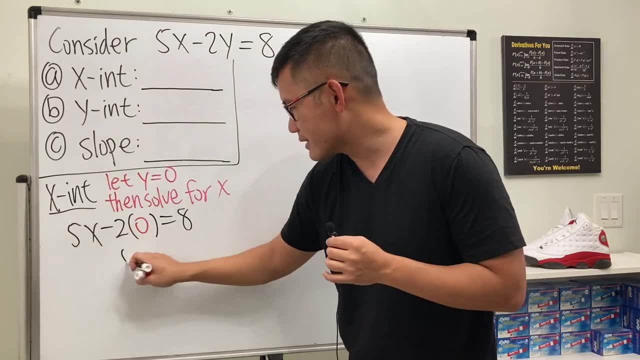 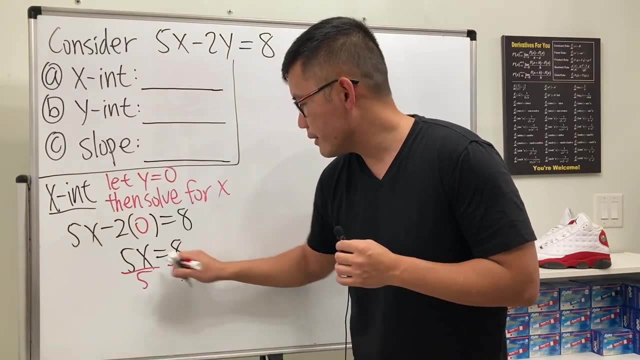 And then this time that will just be 0, so we get 5x equals 8, and this means 5 times x is equal to 8.. Therefore we divide both sides by 5,, they cancel, and we have x is equal to 8 over 5.. 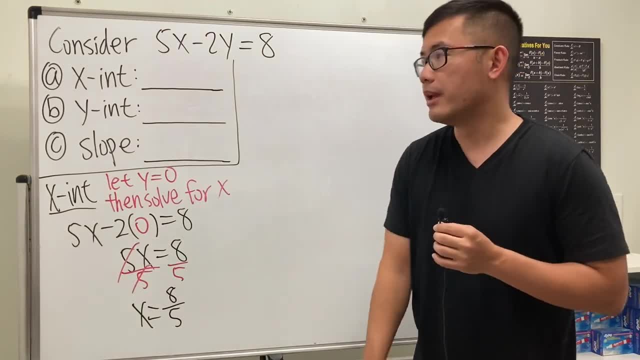 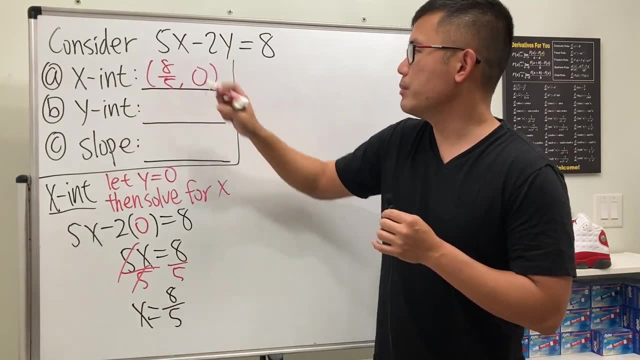 So this is the x-value for the x-intercept For the answer. I would like to write it as 8 over 5, comma 0, because this is the point. This is the x-value and it also shows us that the y-value for the point right there is 0.. 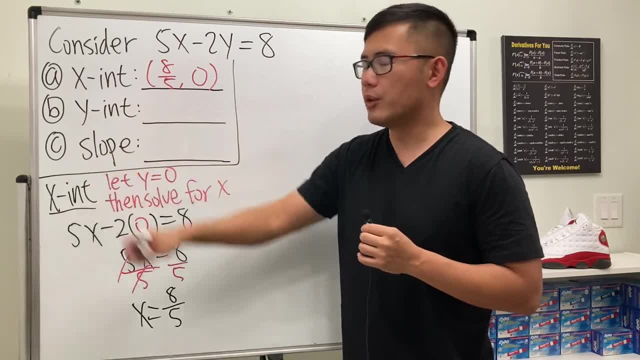 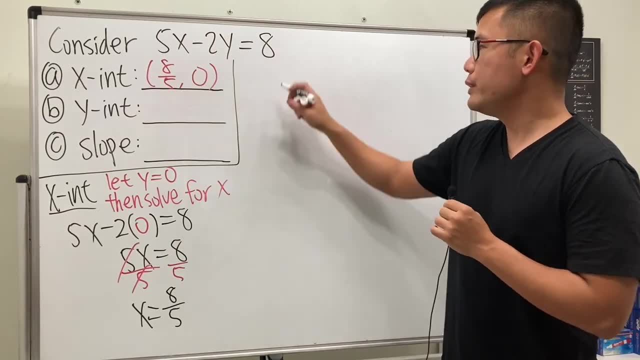 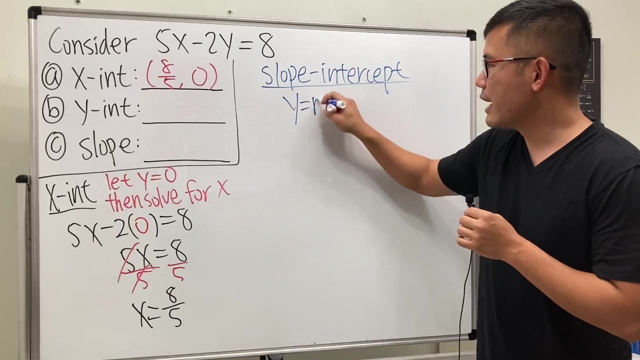 Next we will do the y-intercept and actually the slope at the same time. Here this equation: it's in the standard form. We don't like it. The y is the so-called slope-intercept form of the line, namely y equals mx plus b. 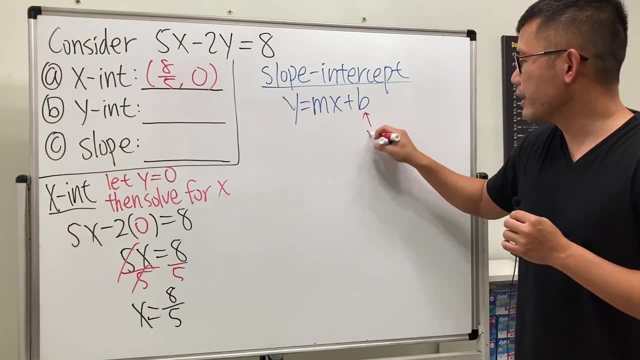 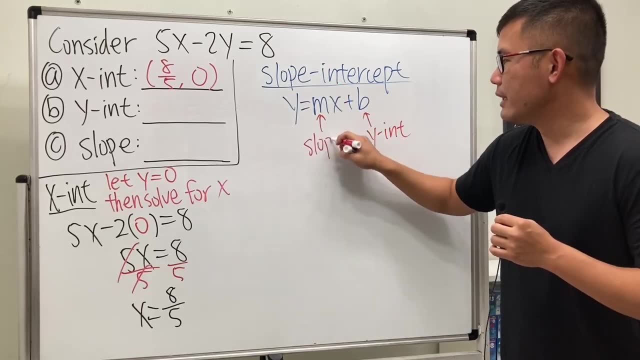 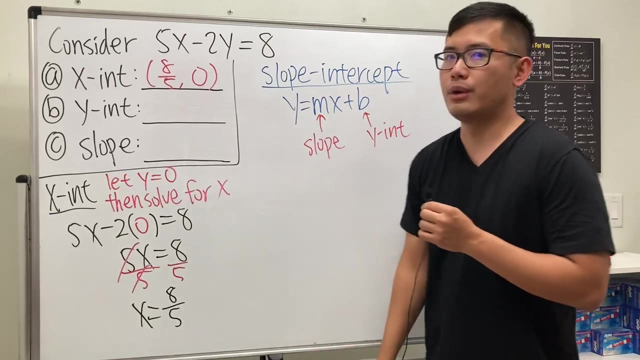 The b. right here is the intercept, and more precisely this: right here is the y-intercept, And then the m. right here it's the slope. So the idea is, if we can write this equation into this form, then we'll be able to answer c and b right away. 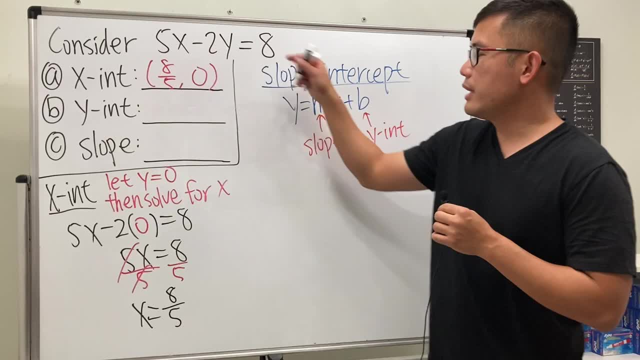 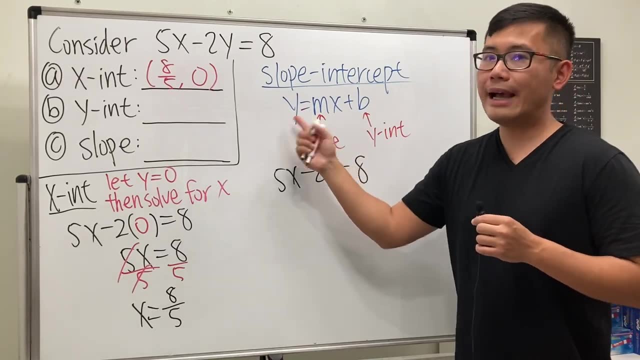 So let's just go ahead and make that happen. Let's look at this equation again: 5x minus 2y equals 8.. Well, in order to get to this form, we will have to isolate the y, which is right here. 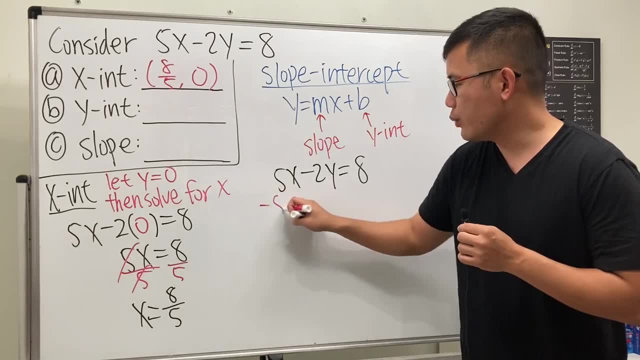 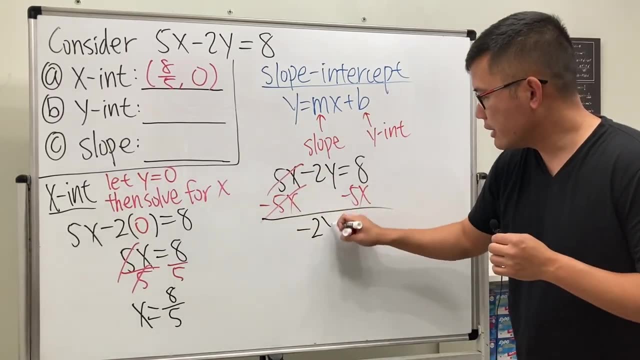 That means we should move the 5x to the other side, and we have to do that by minusing 5x on both sides, And then, right here, minus 2y, bring it down and that's equal to negative 5x, and then plus 8..